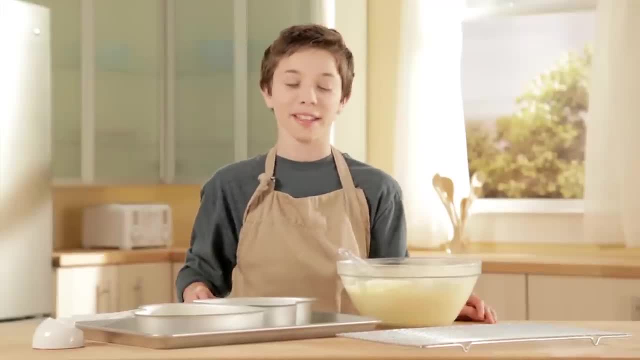 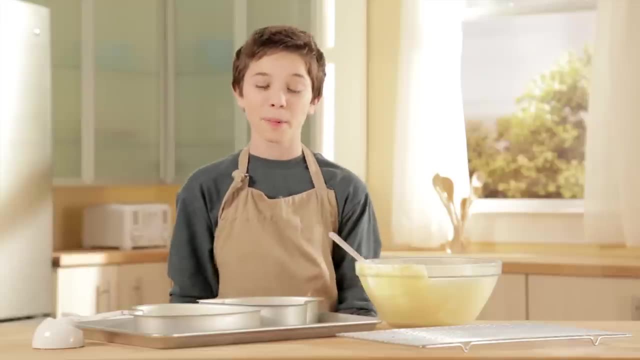 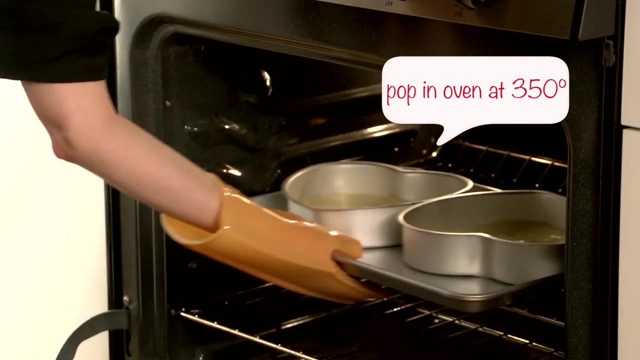 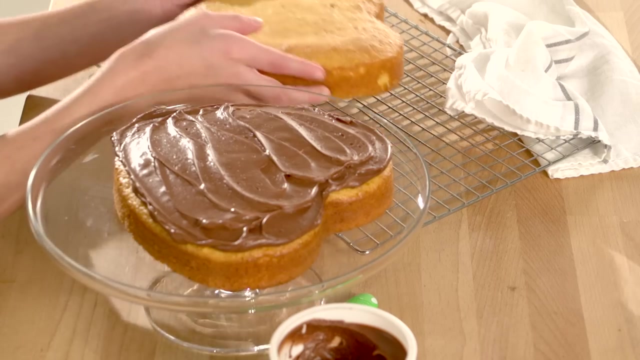 Now that the batter is mixed, I'm going to pour it into this 9-inch pan that I've already sprayed. Now we'll tap it on the counter to get rid of any air bubbles. I put a layer of frosting in the middle so I can stack this one on top of it. 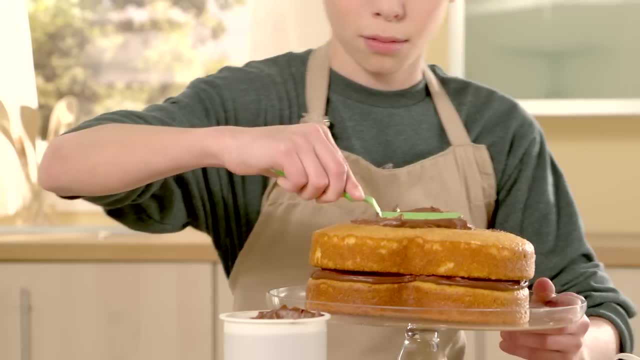 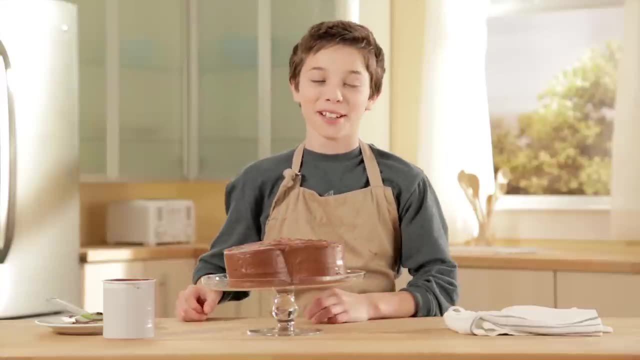 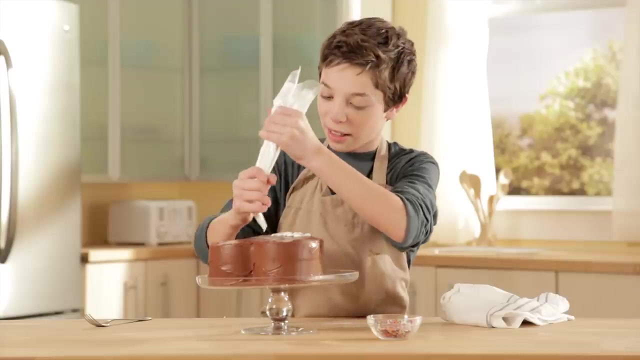 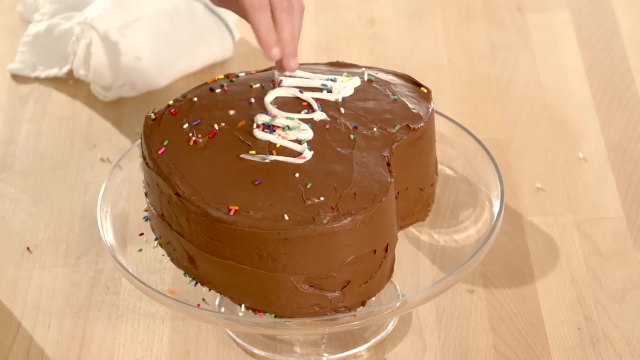 Now it's time to frost the cake. Make sure to get all the little spots too. Now it's time to decorate. She'll love this. I'm using vanilla icing. And now for the finishing touches: Sprinkles, Ta-da. 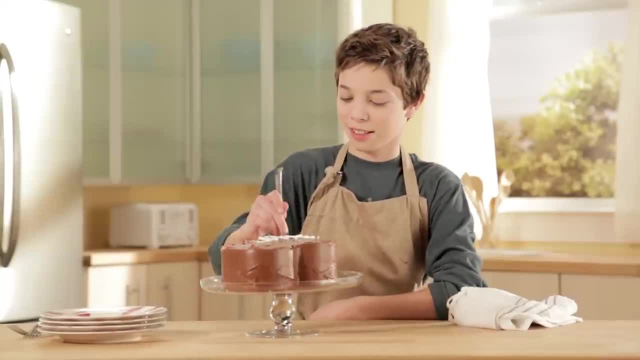 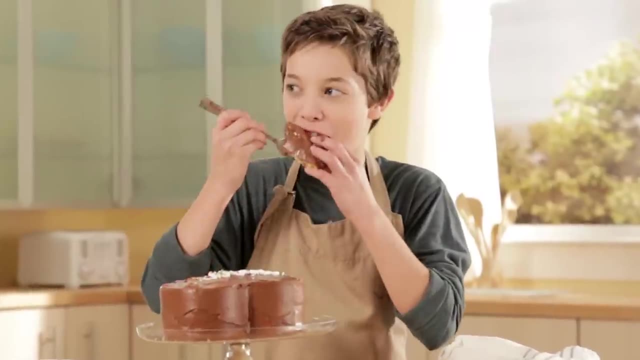 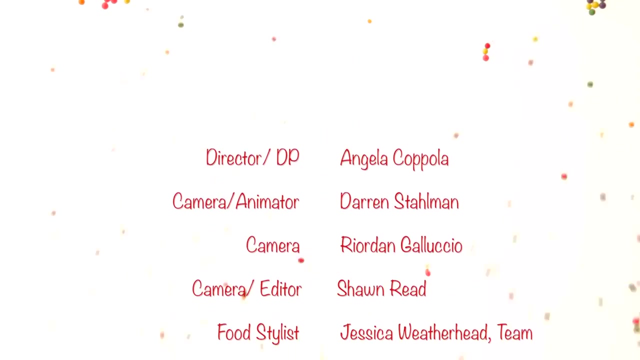 Maybe she won't notice if I just take a little piece. Oops, Looks like I have to make a new cake. Thanks for watching and I will see you next time. Bye. 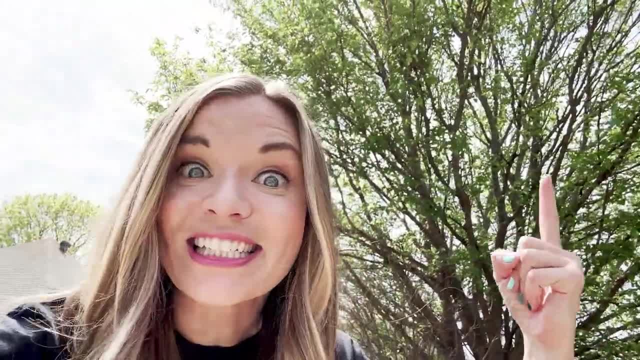 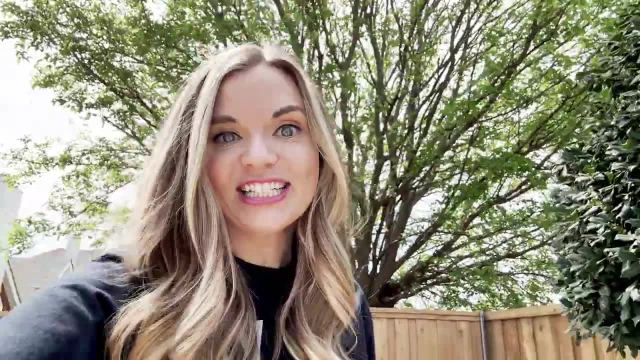 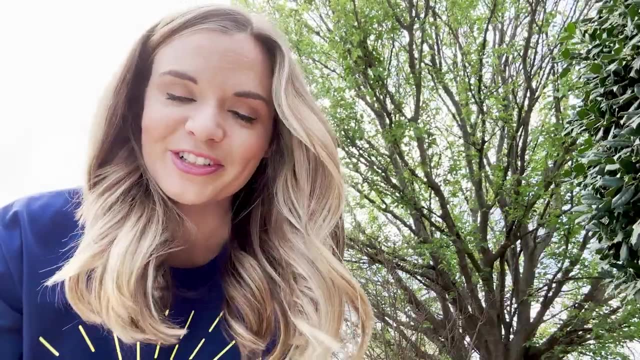 Holy mackerel, You can cook with energy from the sun. In today's episode, we will be assembling a solar oven, cooking with it and learning all about the energy it takes to make it work. It might surprise you that sunlight on its own isn't hot Solar energy. 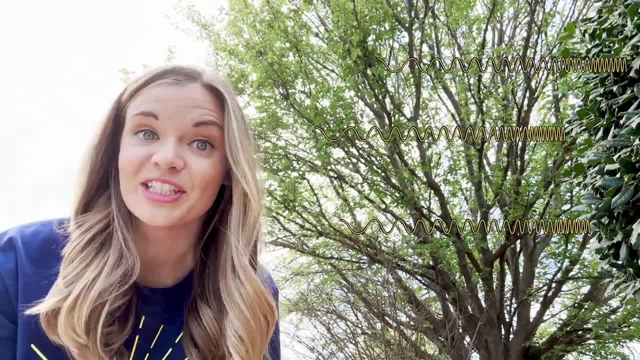 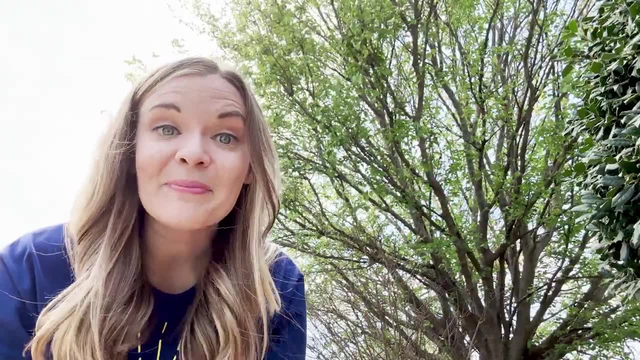 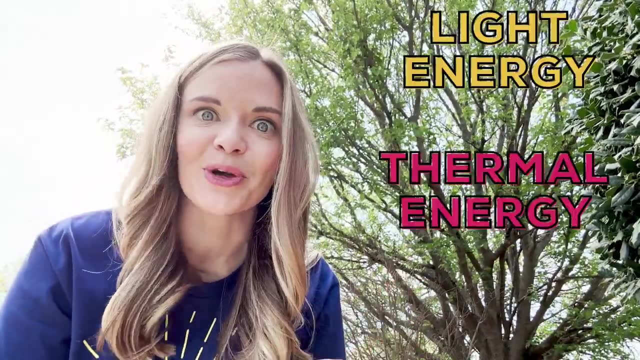 or energy from the sun travels in waves or is radiant energy. It takes about eight minutes for light to travel from the sun to the earth. That same energy is transferred to air molecules in a method known as radiation, which converts light into thermal energy. This is hopefully what 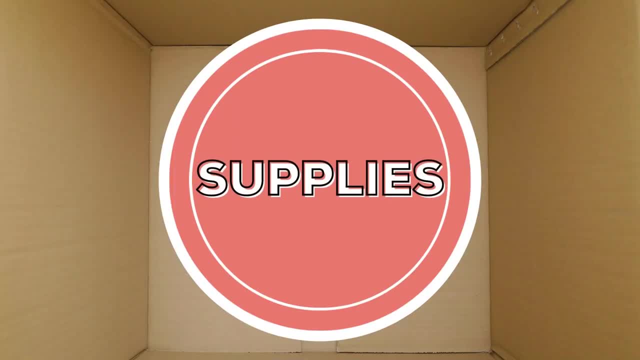 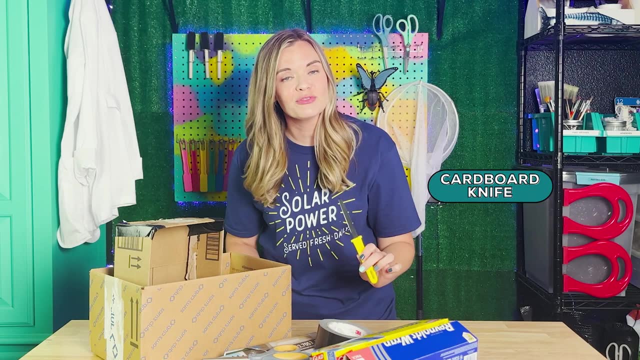 we can get to happen in our solar oven today. Here are some supplies you may need: Cardboard boxes, newspaper, some heavy-duty tape, scissors, a cardboard knife or a box cutter. This is a little more kid-friendly. Plastic cling wrap, aluminum foil, instruction paper.